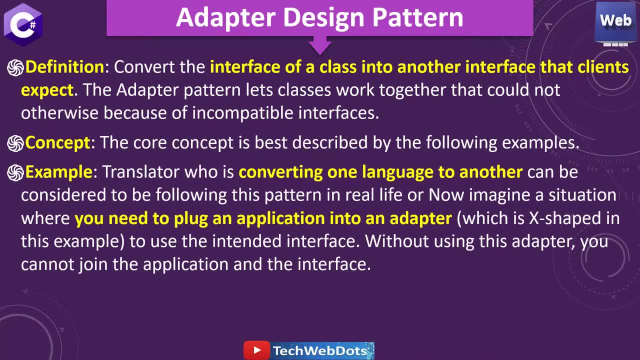 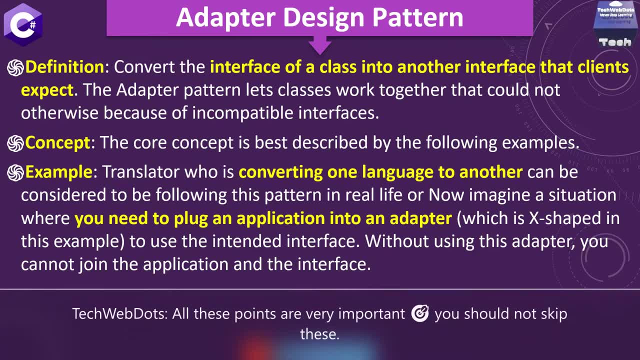 So what is the actual concept of adapter design pattern? Let's first go by example. For example, translator, who is converting one language to another, can be considered. Now imagine a situation where you need to plug an application into an adapter where X shape is the example to use the intended interface. 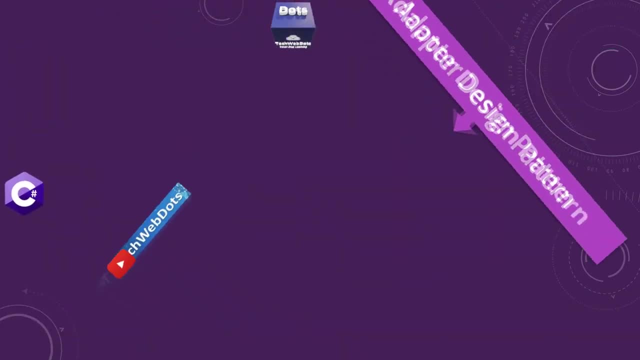 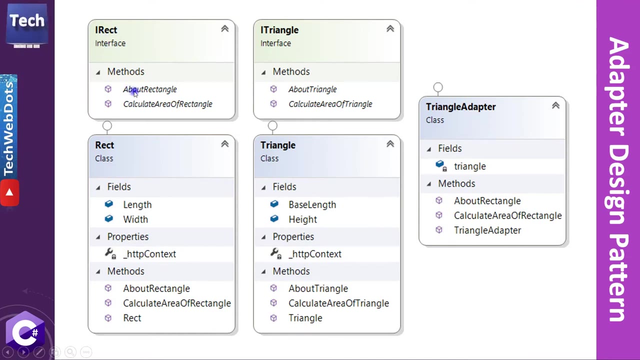 Without using adapter, you cannot join the application. So let's have a look of the class diagram that I am going to discuss with you. So this is I-Rect interface. It contains two methods about rectangle and calculate area of rectangle. 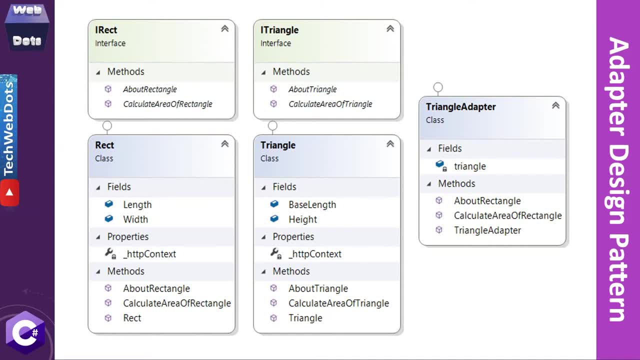 If you are not from the mathematical background, then don't worry. This is a very simple example. It doesn't require the mathematical background and I will explain you in very basic way. Now, if I talk about the Rect class, which is implementing this I-Rect interface, 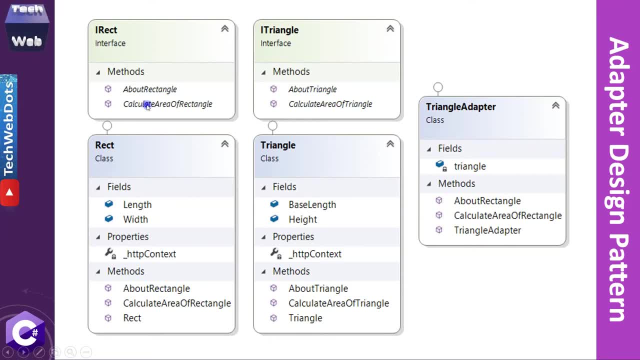 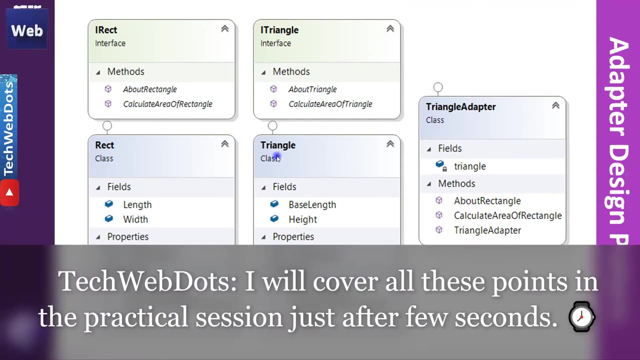 So, simply, we are specifying the detail of about rectangle, The calculate area of rectangle, and with two properties: length and width, which is required, obviously, and HTTP context we are using to write to the response. In a similar way, we have I-Triangle interface and triangle class, in that we have base length and height, which is required to calculate the area of triangle. 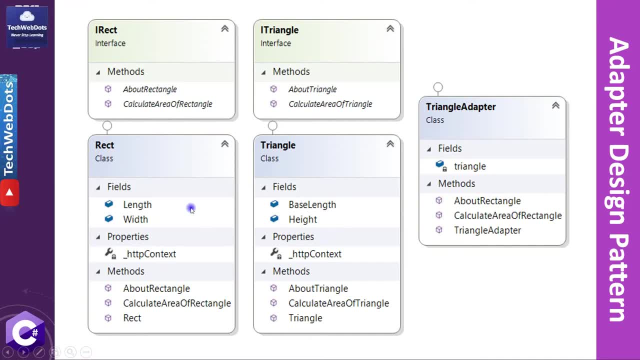 And, similarly, we have one property and two methods that we are implementing Now. the third one is a triangle adapter, which is actually playing an adapter role To inject into the application, and we can use that. Now it's time to see all these things in action. 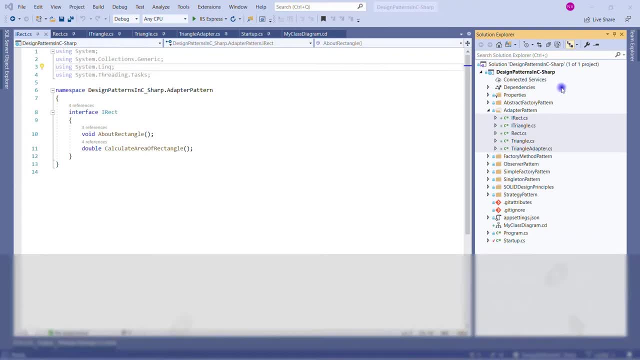 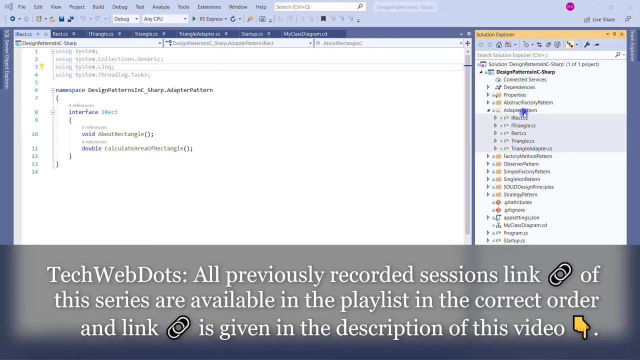 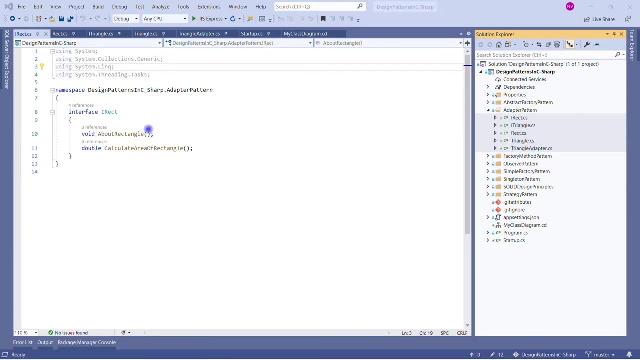 Let's switch to Visual Studio. As you can see, this is the simple ASPNET Core empty web application that I was using in my all the design pattern sessions, And here you can see there are five classes: I-Rect, I-Triangle, Rect Triangle and Triangle Adapter. 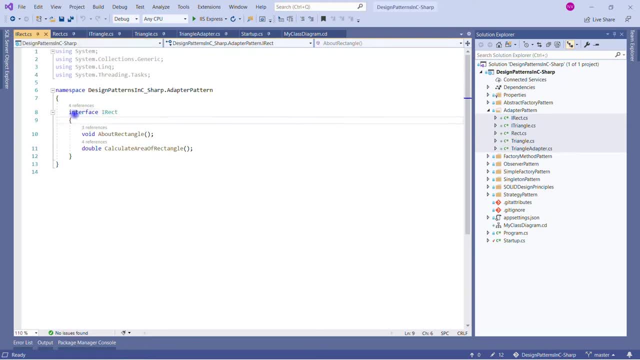 So we will discuss one by one. The very first one is I-Rect, in that what we are specifying, there is an interface I-Rect And there are two methods. So we will discuss one by one. The very first one is I-Rect, in that what we are specifying, there is an interface I-Rect, And there are two methods. 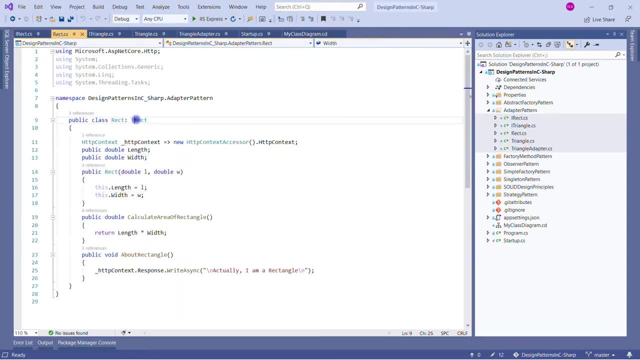 And in Rect class we are implementing this I-Rect interface And in its constructor we are initializing the length and width of this rectangle. And in another two methods we are simply printing a message onto response. And in calculate area of rectangle we are just multiplying length into width. 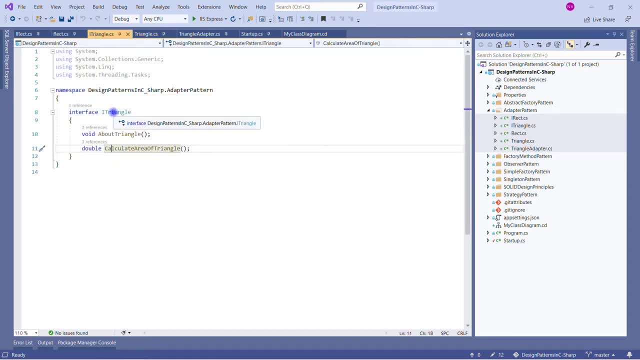 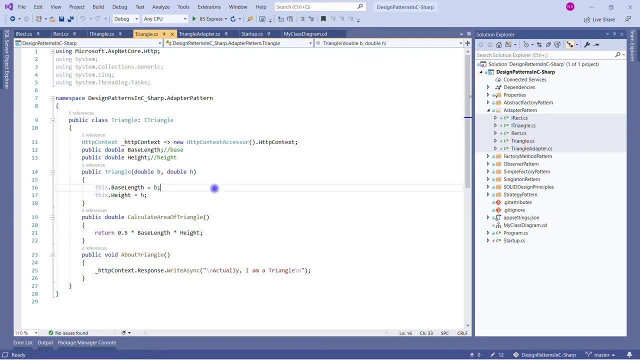 And the same case is for triangle. We are creating a one interface, I-Triangle, And there are two methods: One more triangle And then another triangle, And the third method is a triangle class which is implementing I-Triangle interface. 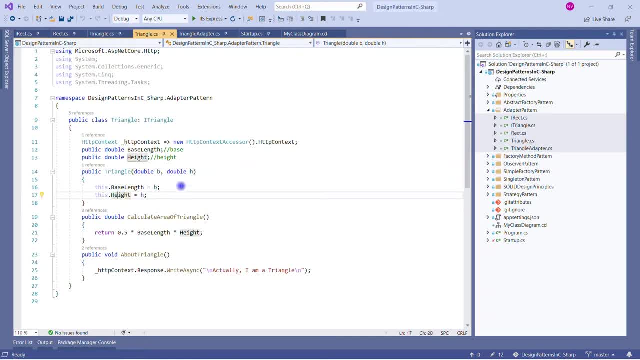 Okay, And using this HTTP context to write to the response. And base length and height is actually required to calculate the area of triangle. Okay, So we are multiplying 0.5 into base length, into height, And simply in above triangle we are displaying actually I am triangle and in rectangle we are simply specifying actually I am rectangle. 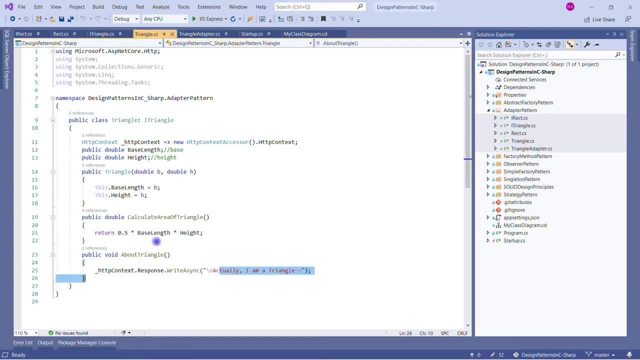 Okay, Now we can simply create the object of this triangle class and easily calculate the area of triangle. okay, but the problem is, if we really don't want to use this I triangle interface, then how can we do that, directly or indirectly? okay, so we will see. 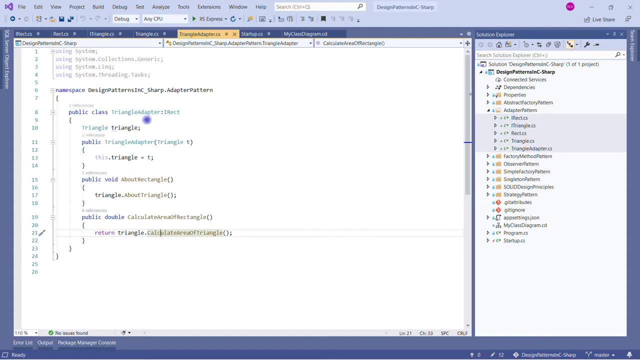 that with the help of triangle adapter. so what we are doing in this triangle adapter class- this is very important and this is the actual idea of this adapter design pattern- in this triangle adapter, we are implementing Iرك interface and you can see, here we are creating the variable of type. 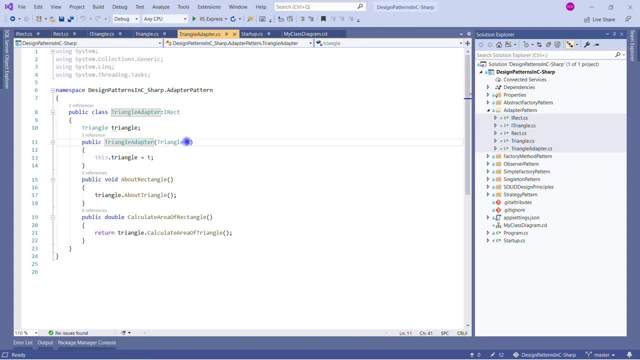 triangle and in its constructor we are getting the variable of type triangle and we are assigning it. it means my triangle adapter is initiated with this triangle variable because we are implementing I rectangle interface- what we are calling here about rectangle, not triangle. okay, because of this, I rect interface a. 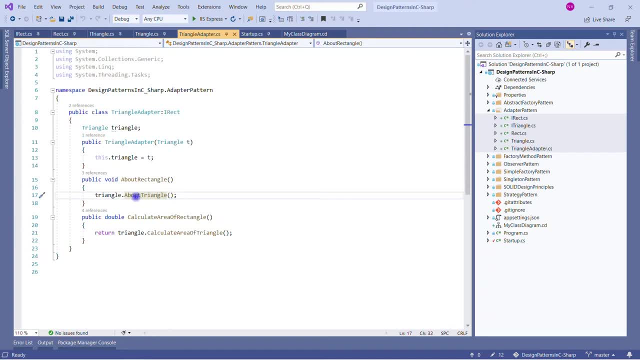 that what we are calling triangle dot above triangle. it means it will go for the triangle class and call this method above triangle. okay, this is how it's going to work and for the calculate area of rectangle, but actually we are working for triangle. we will call triangle dot- calculate area. 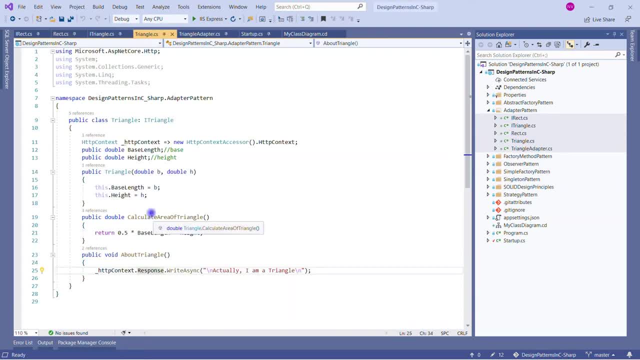 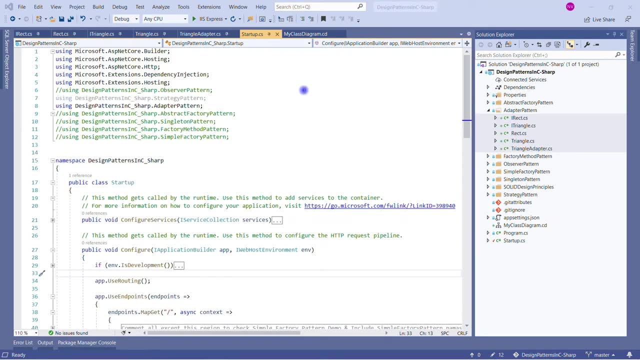 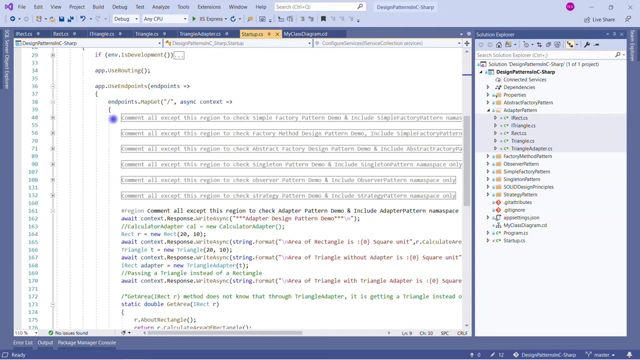 of triangle. now we are calling internally this method- calculate area of triangle. and the last point is how we are calling this. so, as you can see how the solution is working, the required a namespace. i just use it here and comment every other namespace and comment the reason that i don't. 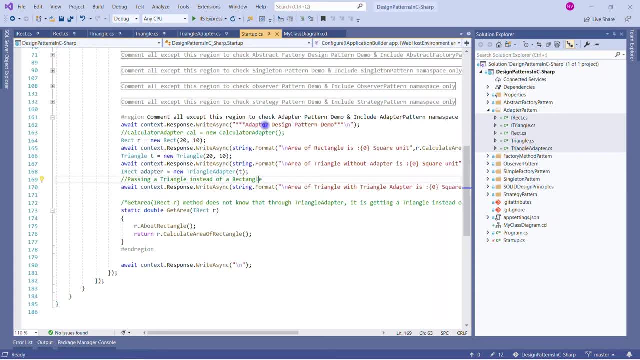 want to use and uncomment the reason that i really want to use. so this time i uncommented the piece of code that i really want to use with this adapter design pattern. so what i am doing here just writing the print adapter design pattern demo onto the response and creating a rectangle. 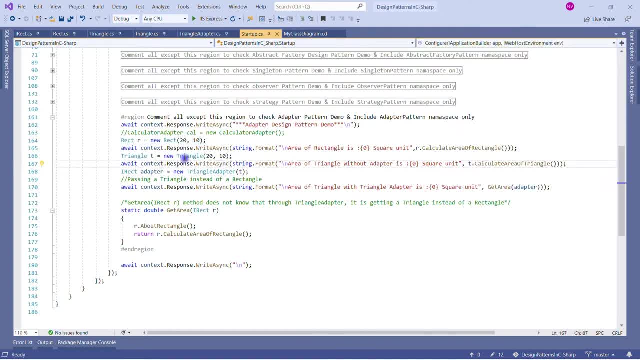 instance and simply calling- let me minimize the screen- and simply calling- r- dot calculate area of rectangle. this will simply return the calculation of a area of rectangle. on my response, then i'm creating triangle instance and calling t- dot calculate area of triangle, and now it will display the area. 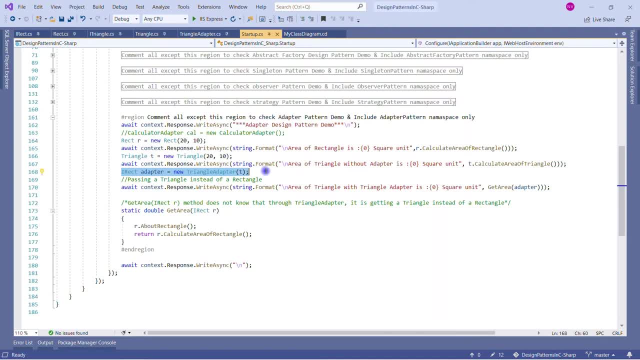 onto the response. but in third line, this is a special case of adapter. what we are doing here in i rectangle we are creating new triangle adapter. okay, because we are already implementing i rect in this triangle adapter class and we are creating a new triangle adapter class and we are 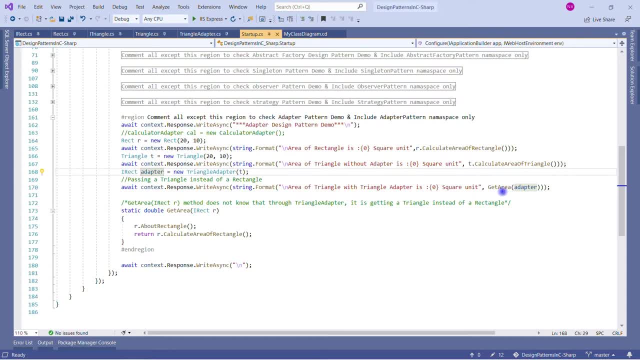 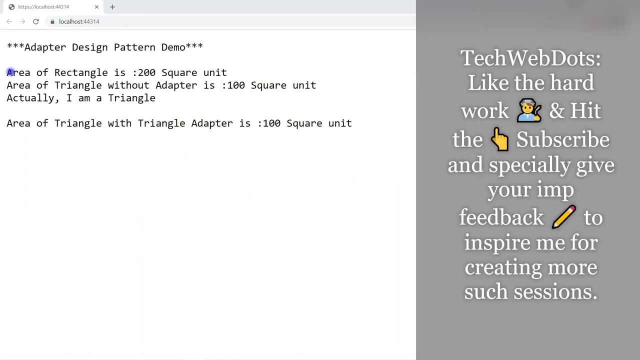 and we are passing this adapter instance to this get area method. so what actually this get area is doing? it is receiving I rect of type variable and from that it is simply calling about rectangle and calculate area of rectangle. let me run the solution now. as you can see, result is expected, area of rectangle is simply. 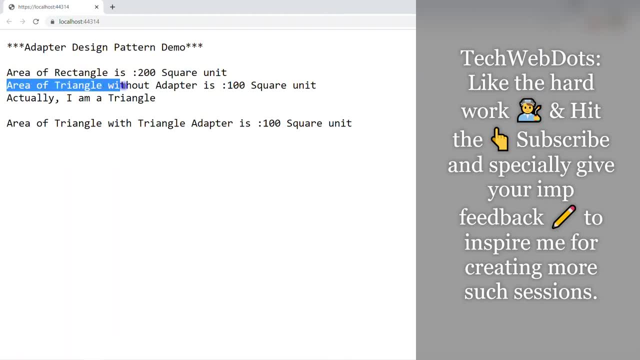 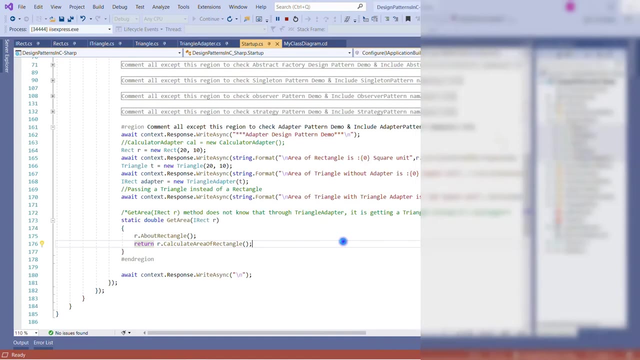 calculated with the help of instance, which is 200, area of triangle is also calculated without adapter- is 100 square unit. but actually, when we are using triangle adapter, then we are also able to calculate the area of triangle, which is 100 square unit. okay, so let's go back to the solution and don't worry if these. 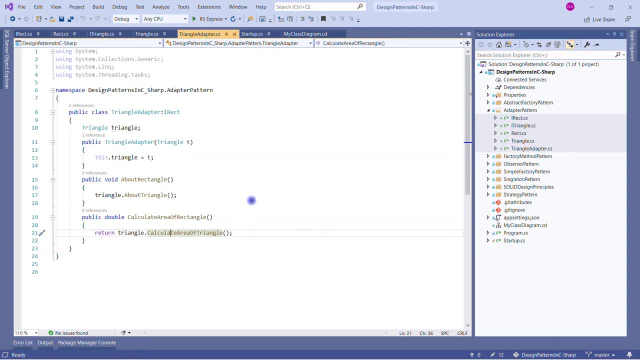 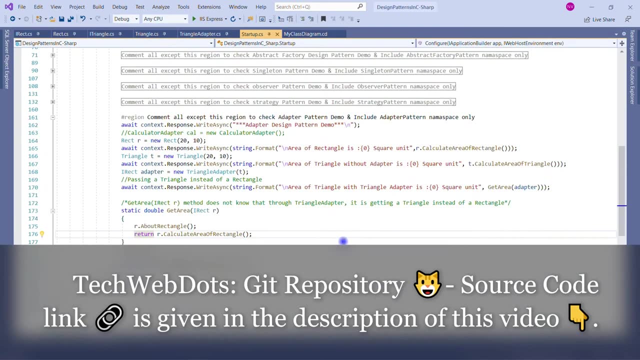 things are still not clear. I will give you more example and I will give you more important points that will be really helpful for you to understand all these things. so don't worry about the piece of code. this piece of code is available in the description below. 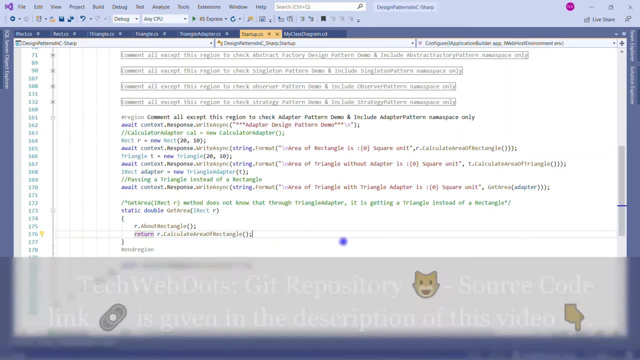 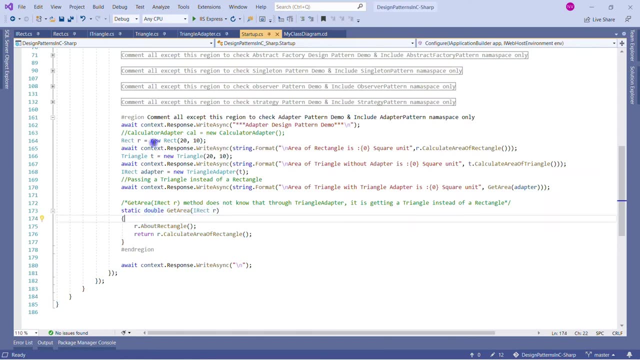 on github repo and the link is given in the description of this video. so let me give you more detail about this get area method, how it's going to work, because it can accept instance of rectangle class as well. it can accept instance of triangle adapter as well, so in this way, this I rect class is working for both. 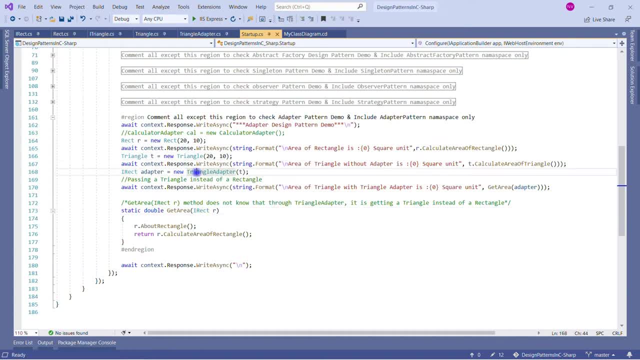 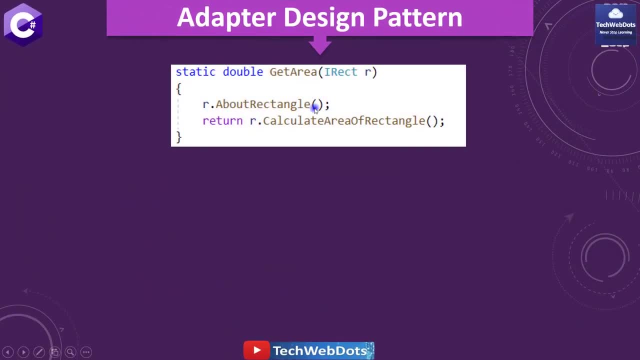 type of calculation. either we are using triangle or rectangle. let me go back to the presentation and give you more detail about this. let's move ahead from here. so, as you can see, this was the main method get area where we are specifying I rect of type R, okay, and we are calling I dot about. 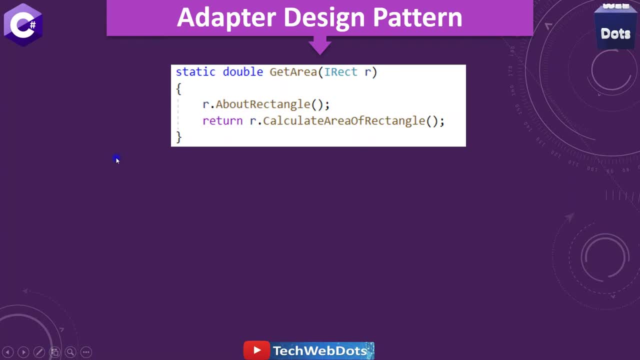 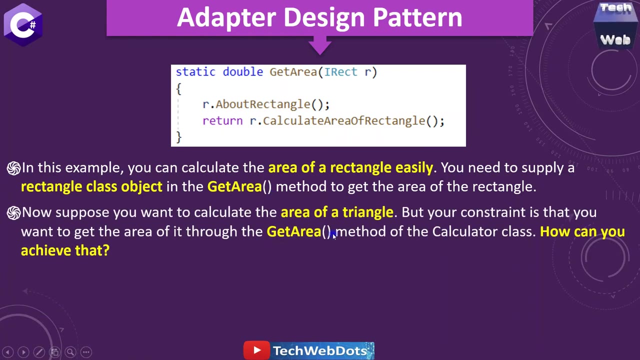 rectangle and R dot calculate area of rectangle. I mean for both the cases, either triangle or rectangle. we are using this method so you can simply calculate area of rectangle easily. so you need to supply a rectangle object in the get area method to get the area of rectangle. but now, if you want to calculate, 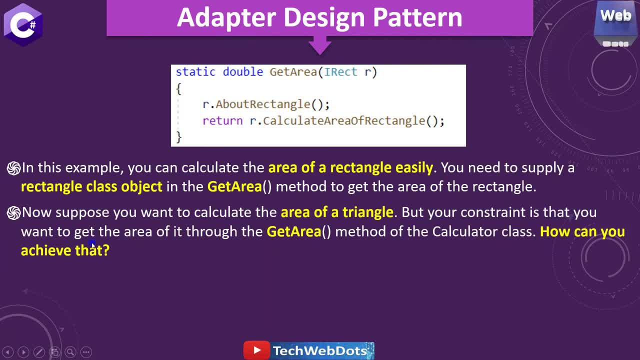 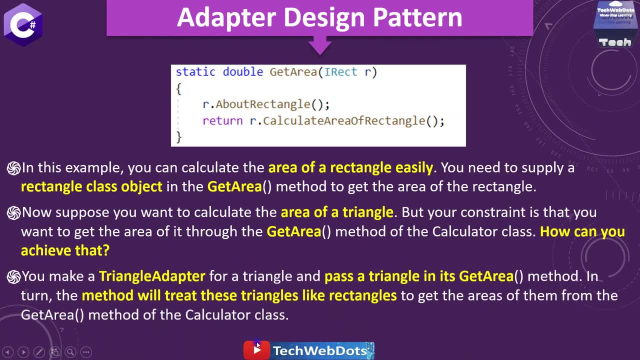 the area of triangle but your construction is not good, then you need to get the area of rectangle by using get area method, because the idea of get area method is that you want to get the area of it through get area only. it means we can use only this method. and how can you achieve that? I just explained. we'll. 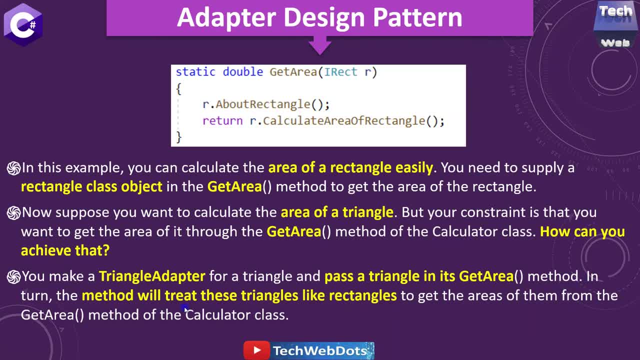 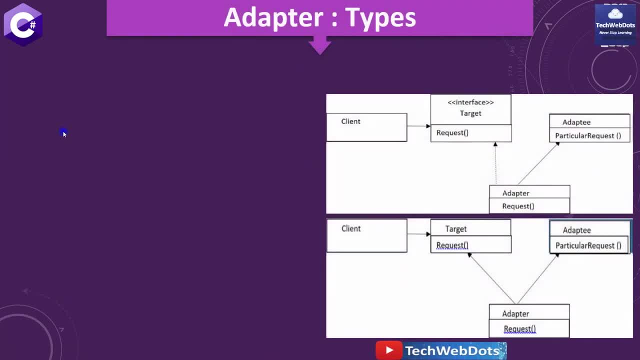 create a triangle adapter for a triangle and pass the triangle adapter in its get area method. in turn method will treat these triangle like rectangles to get the area of them. I hope it is clear now. now let's go back to some few more. So, according to Gang of Four described, two types of adapters are available. 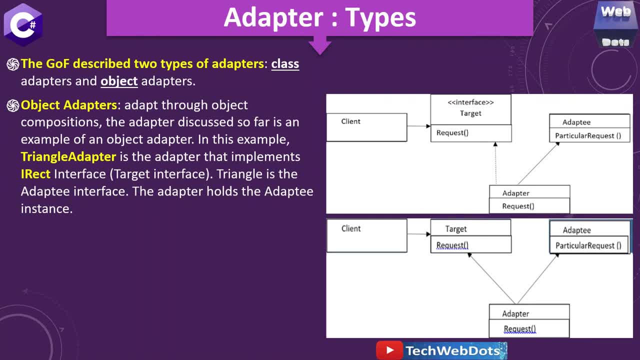 One is class adapter and one is object adapter. So what are object adapters that adapt through object composition? The adapter discussed so far is an example of object adapter. In this example, triangle adapter is the adapter that implements I-Rect interface, which is a triangle interface. 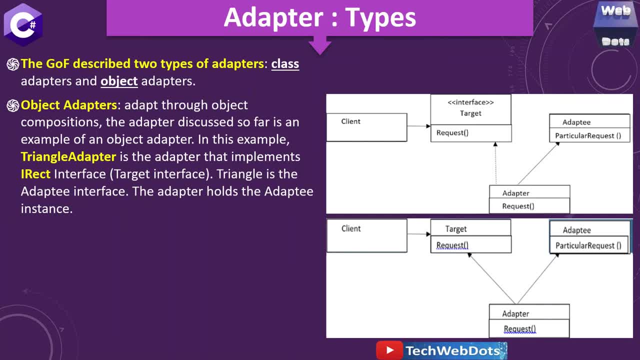 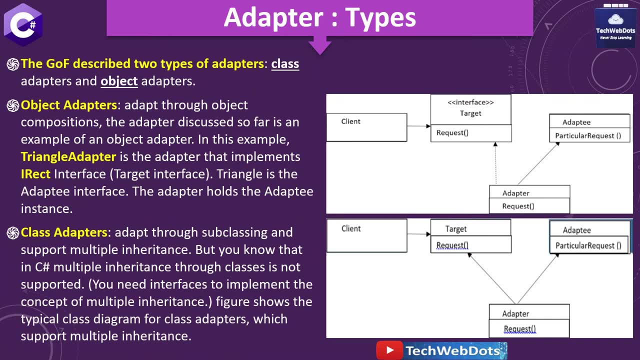 Triangle is the adapter interface and the adapter holds the adapter instance. So that's how the whole concept is working that I just shown you. And the another one is class adapters that adapt through subclassing and support multiple inheritance. But you know that C-sharp multiple inheritance through classes is not supported. 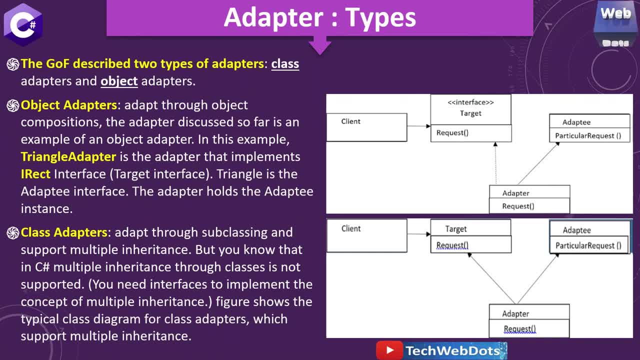 So you need interfaces to implement the concept of multiple inheritance. That is very simple And in the figure you can see the typical class diagram of class adapters which support multiple inheritance. So you can see in this diagram They are target, they are adaptee and they are particular request that we can make with the help of this adapter. 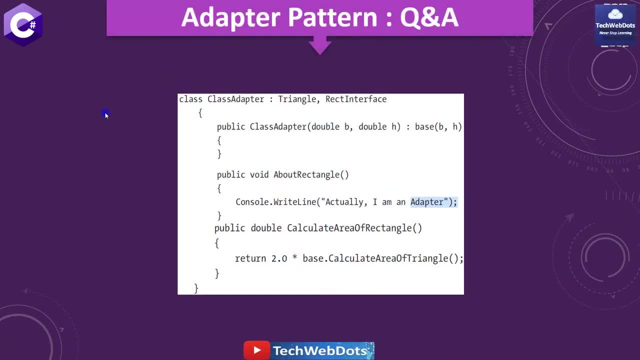 Okay, I hope this point is clear now. So let's go back to few questions and answers. So one question can be: how can you implement a class adapter design pattern? So very simple. We are implementing a triangle class and I-Rect interface. 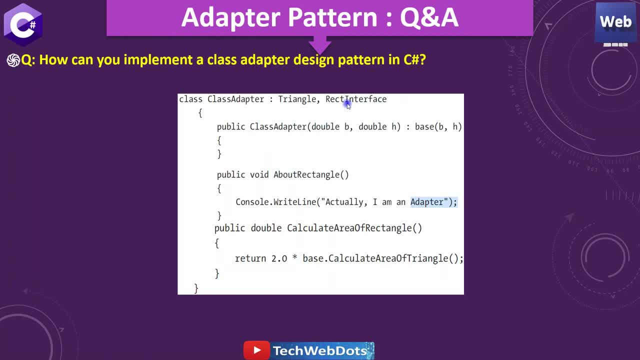 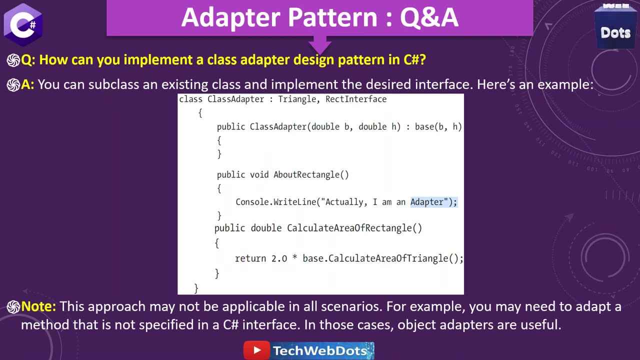 And in that we are specifying the required rectangle interface methods, like about rectangle and calculate, And in this way we can simply use the class adapter. You can subclass an existing class and implement the desired interface with this example. Note: the approach may be applicable to all scenarios. 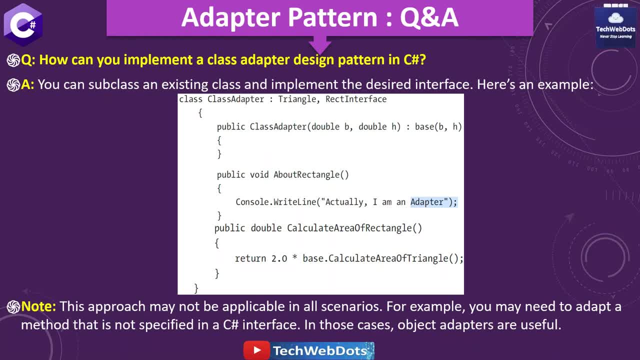 For example, you may need to adapt a method that is not specified in a C-sharp interface, So in those cases, object adapters are very useful. So I strongly suggest you to implement this class interface with your practice and let me know if you face any problem in that. 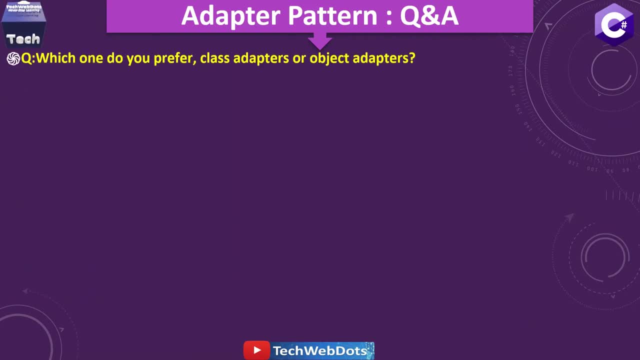 Okay, Let's move on. Let's move to the next question that you might be thinking: which one do you prefer? class adapter or object adapter? So in most cases I prefer composition over inheritance. object adapters use compositions and more flexible. 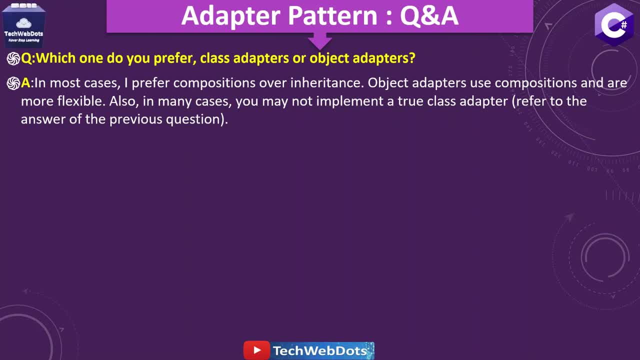 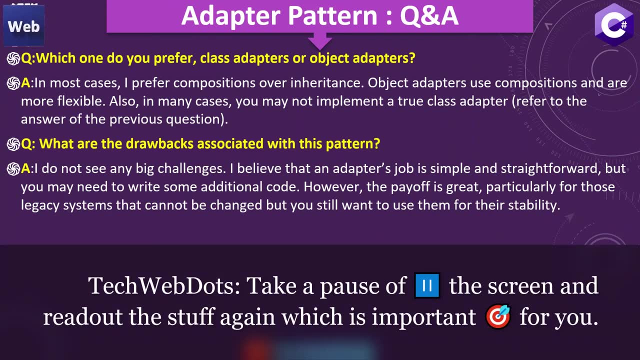 Also, in many cases you may not implement a true class adapter. Refer to the answer of the previous question that I just explained And what are the drawbacks associated with this pattern? So I do not see any big challenge. I believe that adapter job is simple. 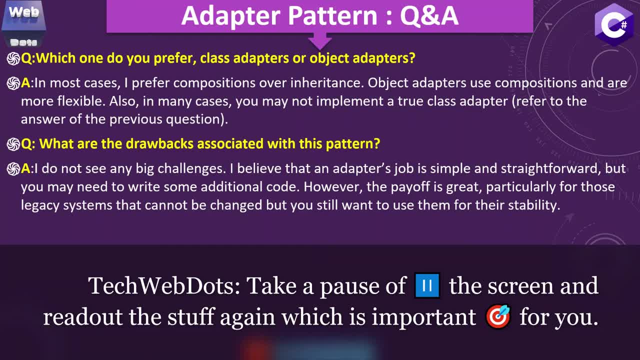 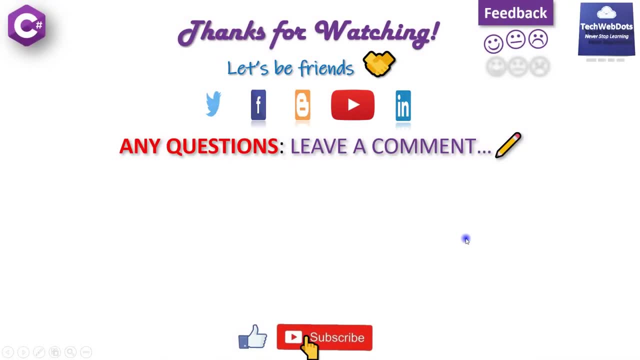 And straightforward, But you may need to write some additional code. However, that payoff is great, Particularly for those legacy systems that cannot be changed, But you still want to use them for their stability. So I hope you like this video. If you have any comment, any suggestion, you can drop into the comment box. 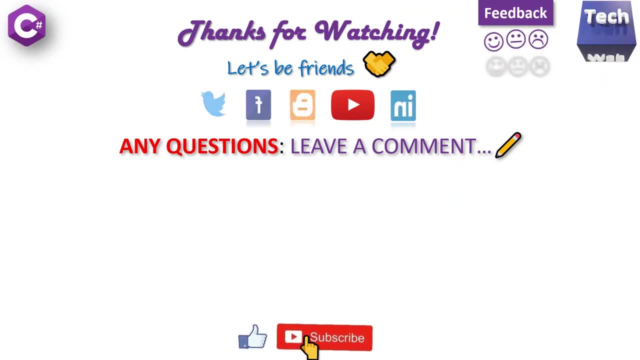 I will reply on that as soon as possible, And your feedback is, as usual, always important. That's the only inspiration for me to create such videos, So I will see you in the next video with some new learning. Till then, bye-bye.